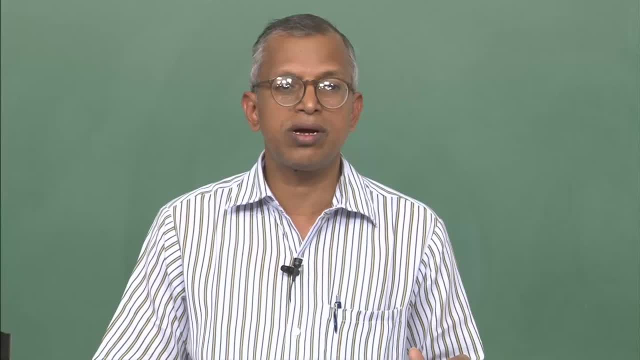 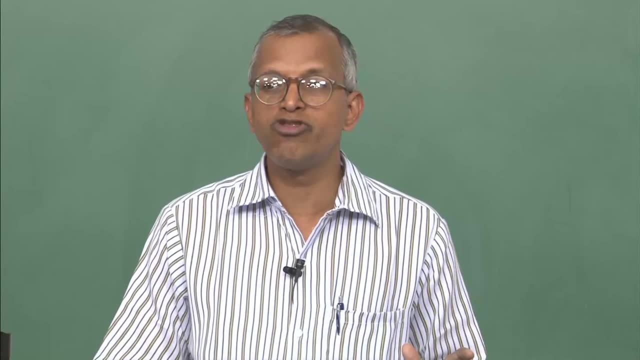 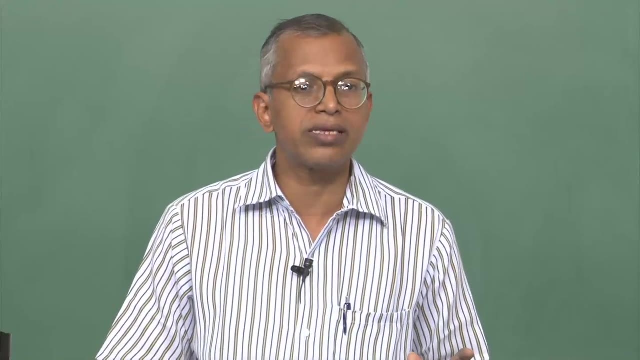 let us recapitulate. If you look at, I started with taking an example where I illustrated how to really determine the activation energy from experiment, provided both are conducted at two different temperatures, And that was a part of an example. Then we moved into the 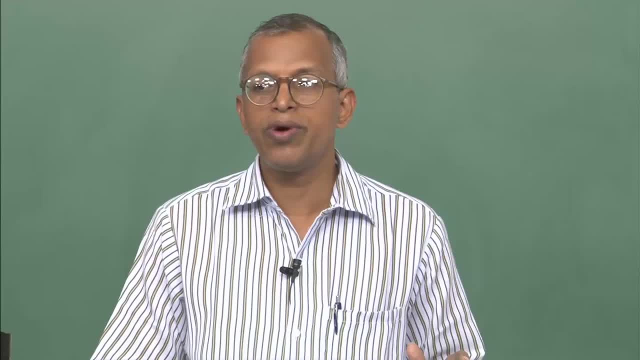 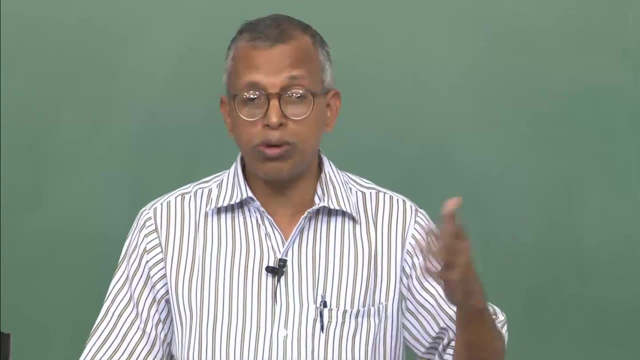 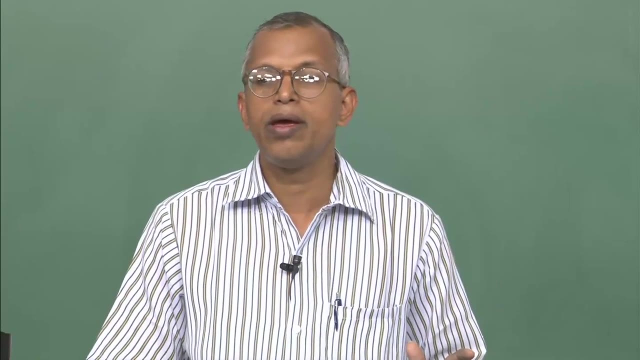 what you call molecular reaction. based on that, we divided, you know, roughly all the reaction into three: unimolecular, bimolecular and trimolecular. Of course quadramolecular reaction can take place, but very unlikely to happen. And then we also define a term known as order of reaction. 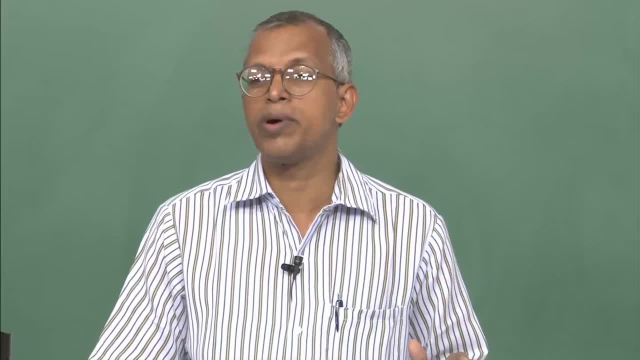 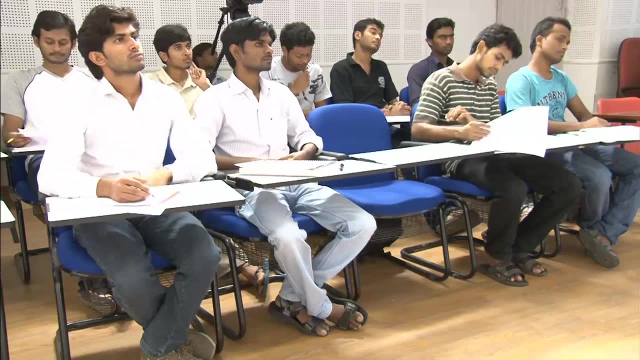 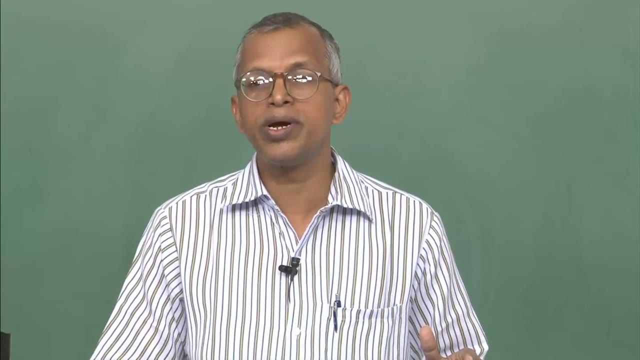 and, based on that, we just, you know, touch upon the first order reaction, second order reaction and third order reaction, Some of the examples I have taken. but, however, if you want to really look at in detail, you need to look at the equations and solve it So that you will see how this reaction rate. 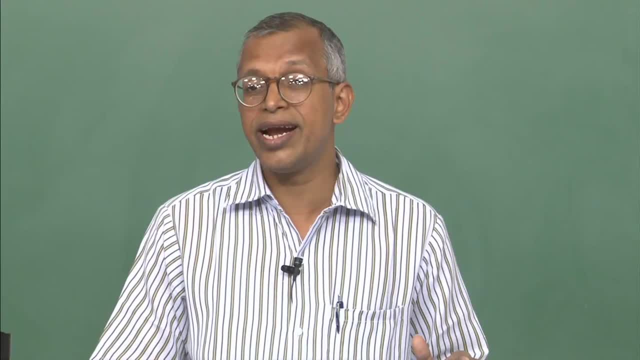 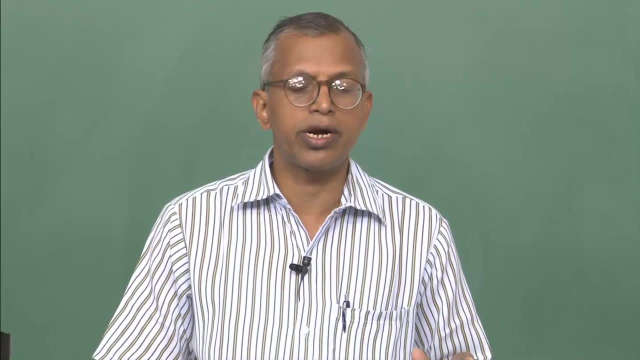 is varying with time. I did not get into that. if some of you are interested, you can look at some standard books on combustion and you can have a feel what it is. Later on, we moved into chain reactions, which is natural in case of fluid. 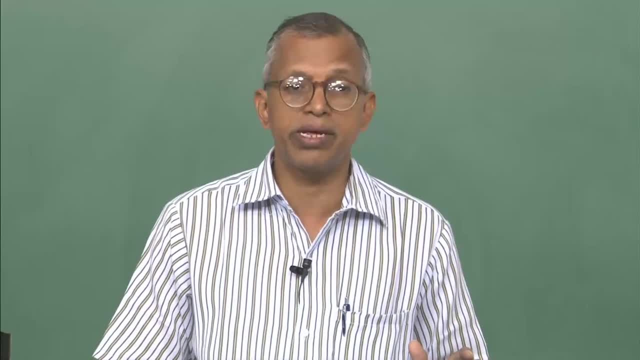 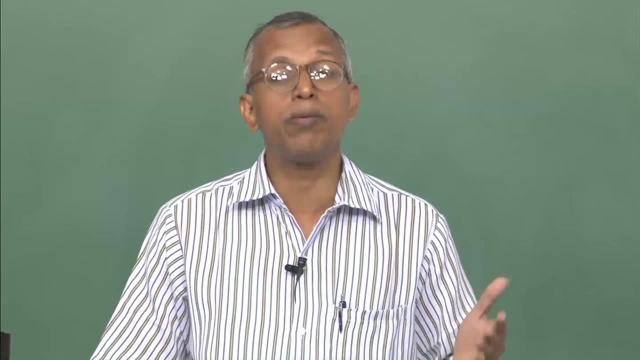 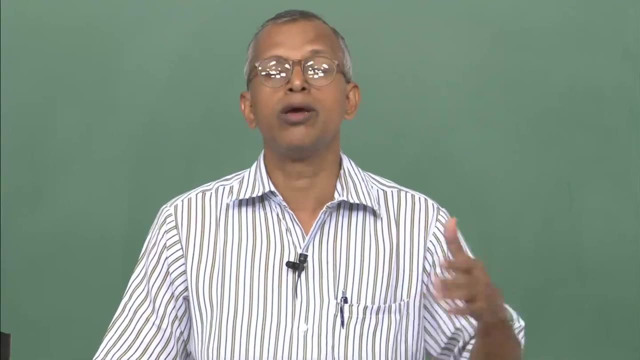 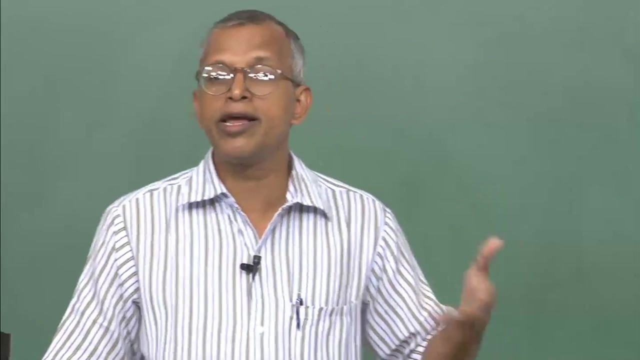 Particularly whenever the combustion reaction is taking place right like chain initiation chain, what you call branching chain carrying reaction chain termination. If you remember, I consider this chain reaction is nothing but a human life, like a baby is taken bar that is initiated. life is initiated and it will be branching, carrying out like learning. 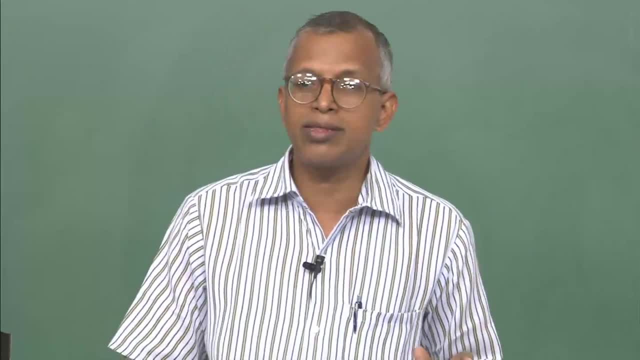 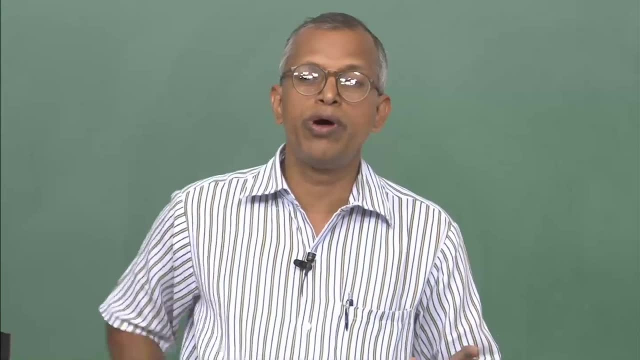 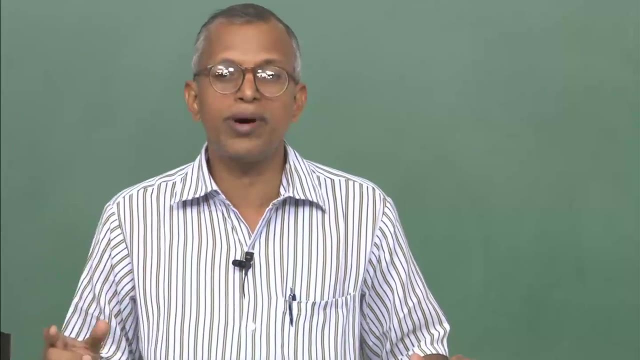 and other things. at the end, you know you will be terminated at the death. So then we moved into the kinetics, the multi step chemistry, you know. I just show you a very glimpses of it just to have a feel how complex it is, not you remember? all those steps involve in the 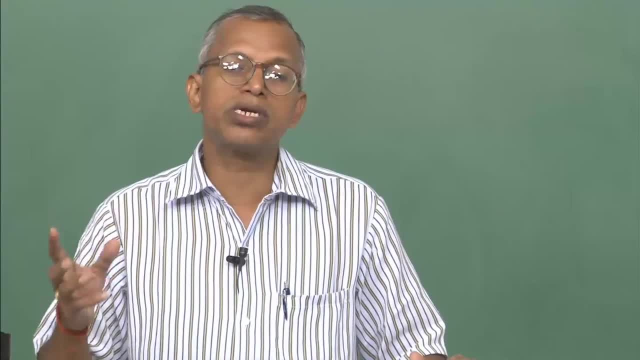 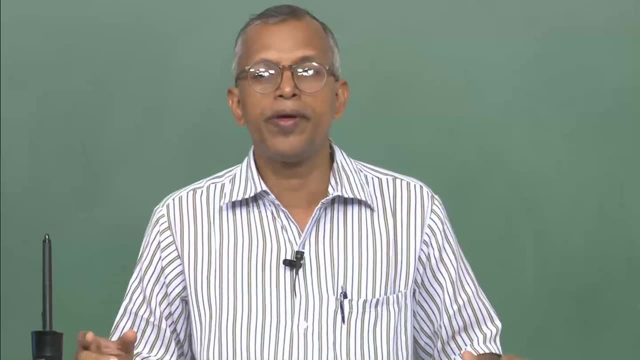 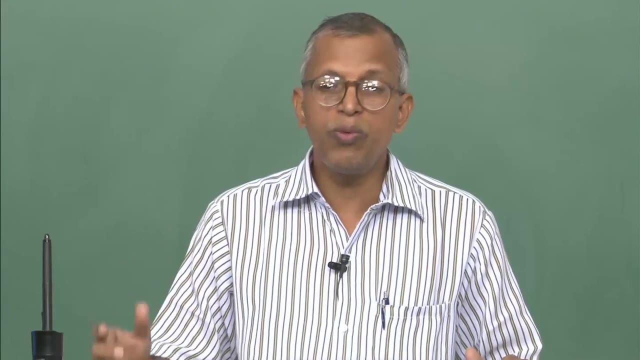 multi step kinetics, But we will be mostly handling with the global kinetics which is, although not occurring nature, it is just a model to overcome the problem of handling multi step chemistry in realistic problem. And then we moved into what you call various modes of combustion, right like flame and 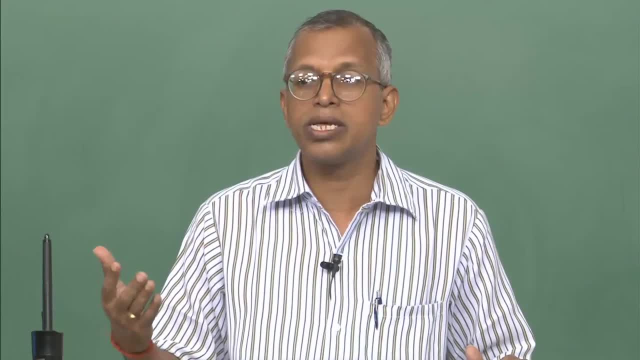 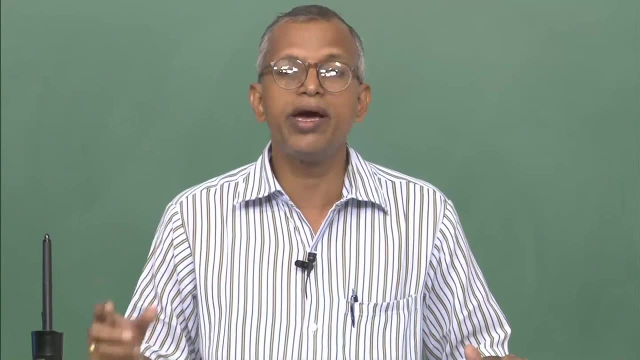 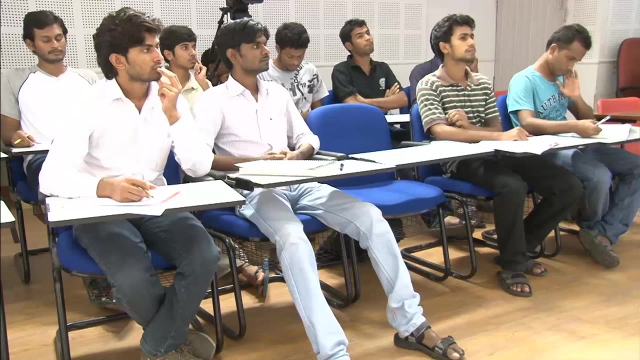 flameless mode. right, and under the flameless mode I talked about smoldering combustion, to just to give you know little bit idea about it. And then we have also talked about premix flame and diffusion flame And, as I told, that combustion is basically a wave right. 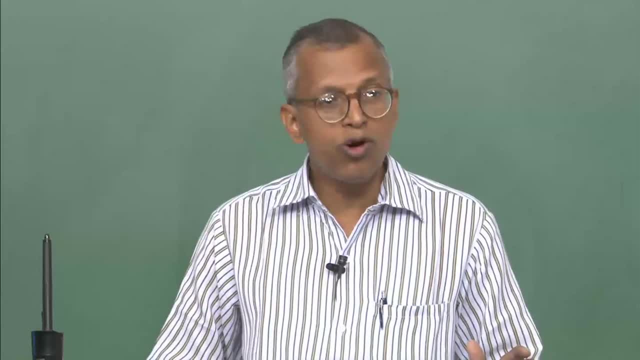 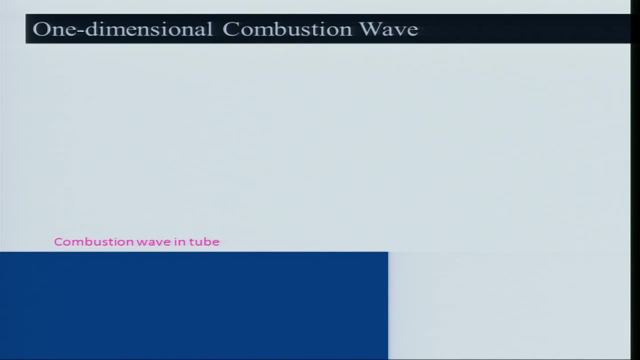 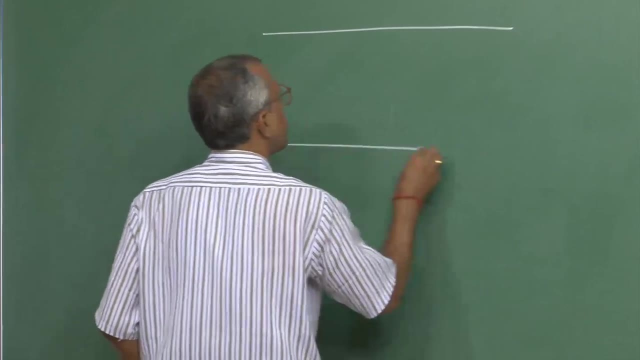 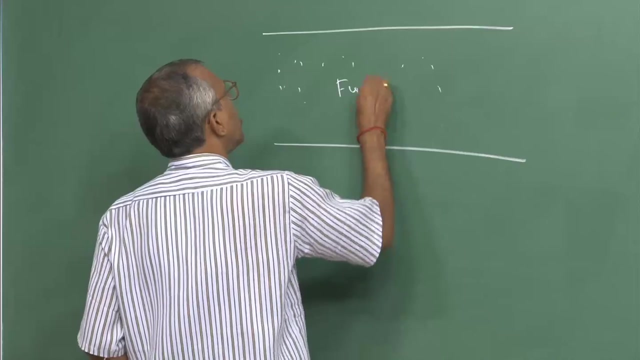 whether it is a wave or not. that we will look at today. it is like your shock wave. it is like a wave If I consider a tube which is mixed with, pre you know, fuel and air. for example, if I take a tube here and this is fuel plus air which are mixed together, right? 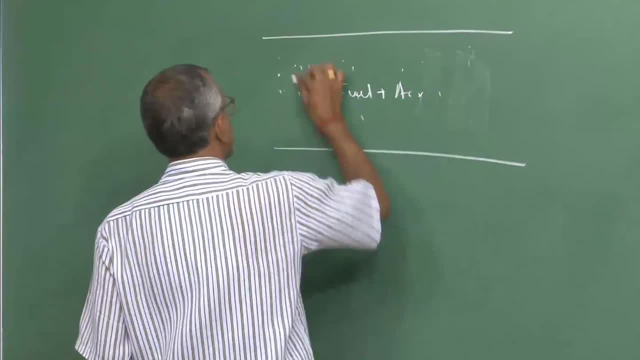 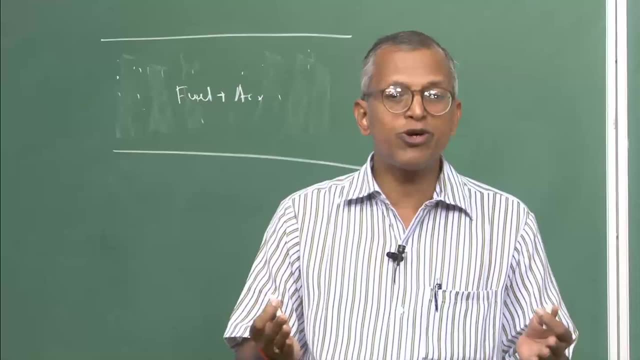 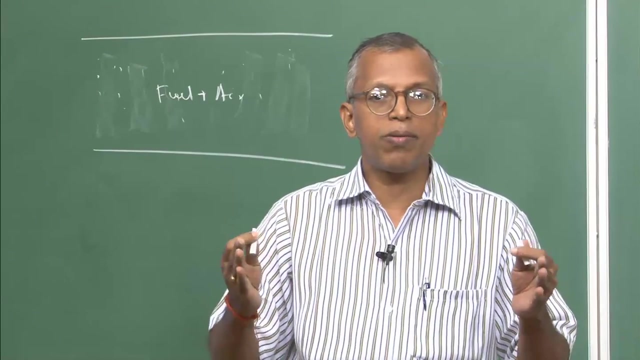 If I ignite- you know these are the mixtures, you know vertical- all mix together, of course, at a what to call particularly fuel air ratio in which combustion can take place, Because we know that there is a two limit, you know, between who is combustion can take place beyond. 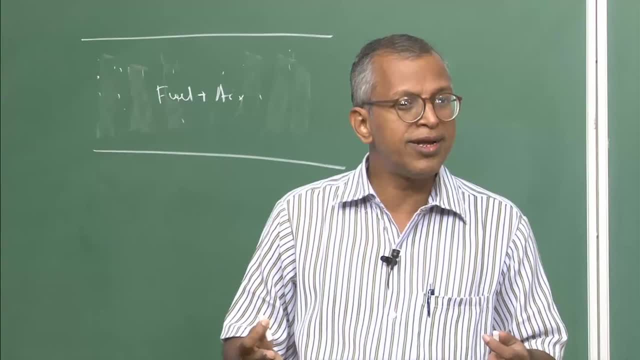 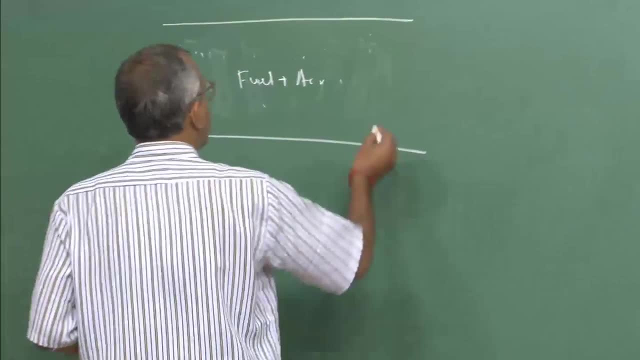 this two limit? it cannot be. Do you know that? what is that limit? that is known as flammability limit. we will be talking about it just briefly. And then that is the fuel air mixture beyond which no combustion will take place. however, 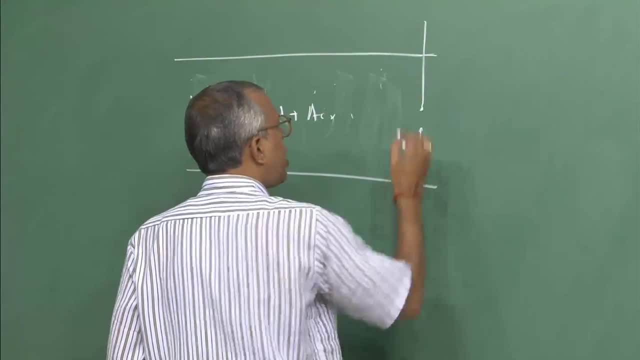 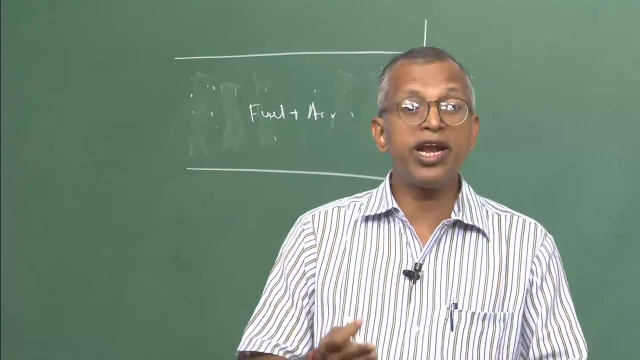 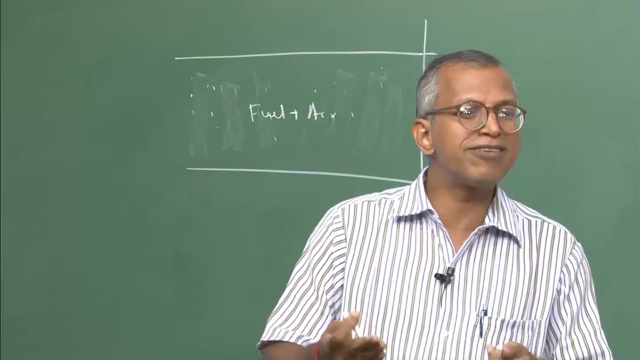 the ignition energy we need to take. If you look at, to ignite something we need to have a flame. to have combustion, we need to ignite it. without ignition can really combustion take place? certainly no initiation is required, So naturally we will ignite. if you look at 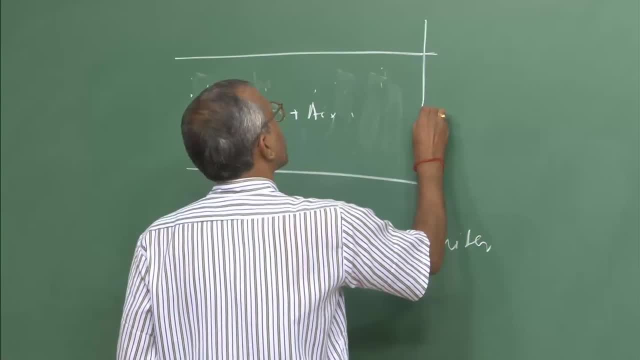 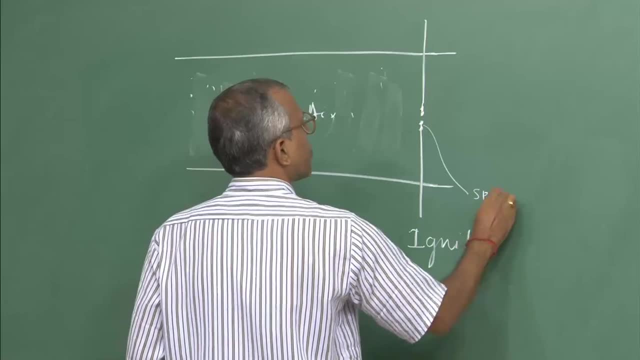 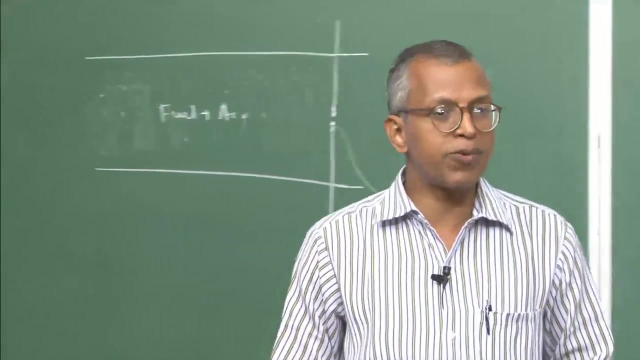 this is igniter, then what will happen? of course this is a spark I am taking about, but with the spark you can say this is a spark plug kind of things. you know, spark plug is one kind of igniter. there are several kinds of igniter as you go along, we will talk about. 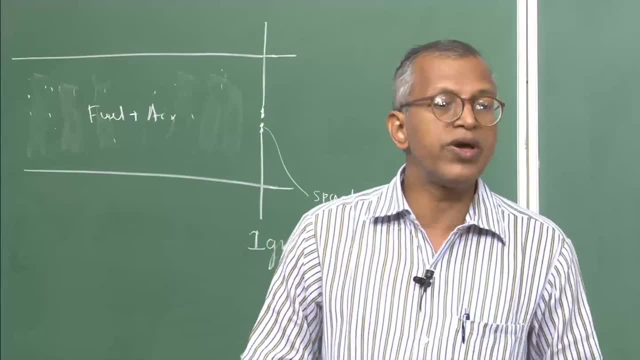 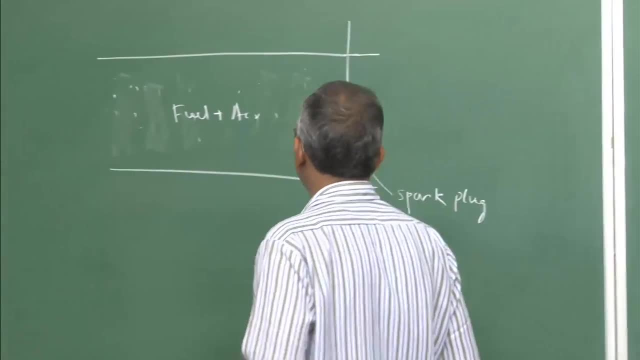 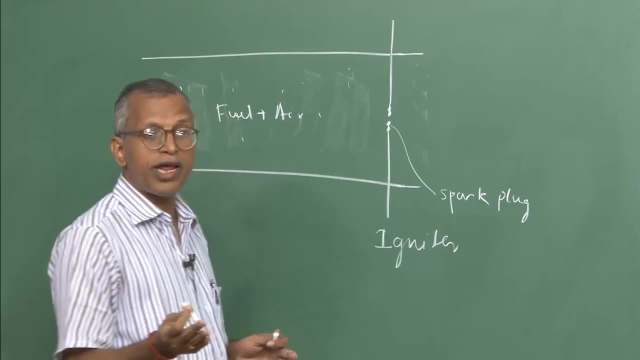 it, particularly in solid propellant combustion, various kinds of igniter you can think of. So if I ignite it, what will happen Here? what will be there? in this place, there would not be any fuel air mixture. will it be there? there might be, but those are, you know, diffusion will be taking place right. 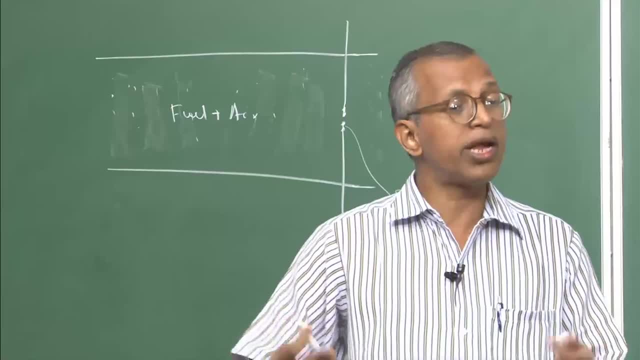 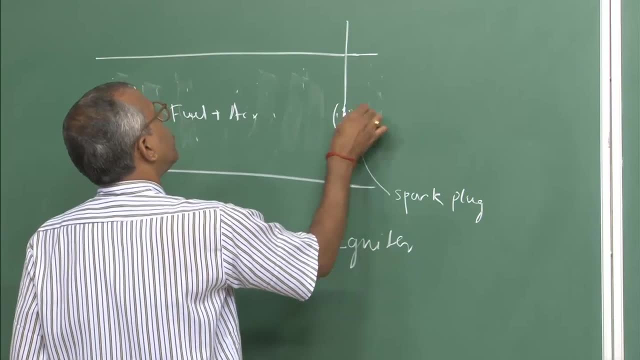 and it will. mixing with air may be below the flammability limit. nothing will happen if I ignite it. So if you look at the flame will be kernel will be coming over here, but it will be moving towards this direction. these are flame, will. 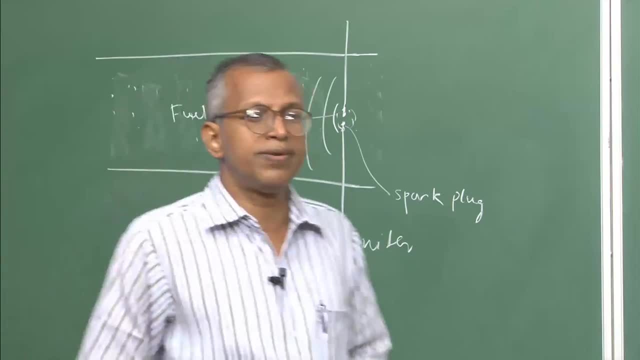 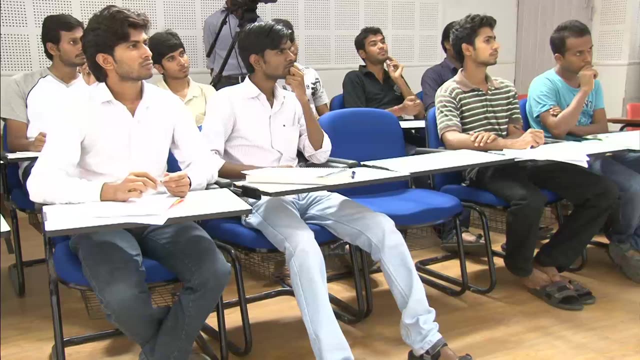 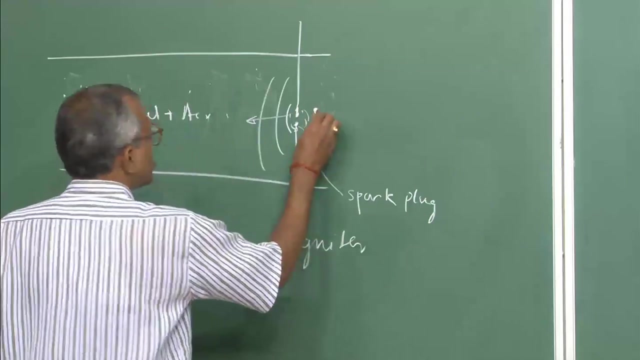 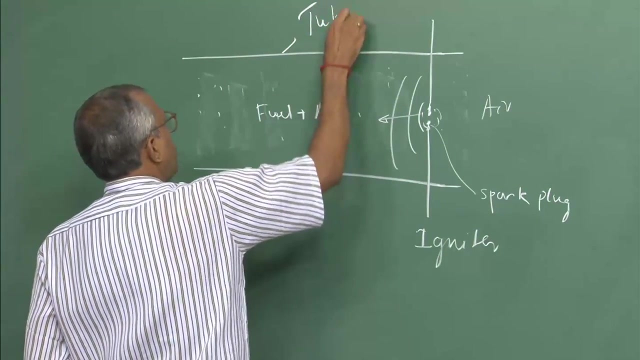 be moving? Will it be moving or will it remain stationary? why it will move? because there is a fuel, air mixture, and which is there on this side, whereas this side it is simply air, right, if this is my tube, this is my tube, right? So this is a simply air which is open to atmosphere am. 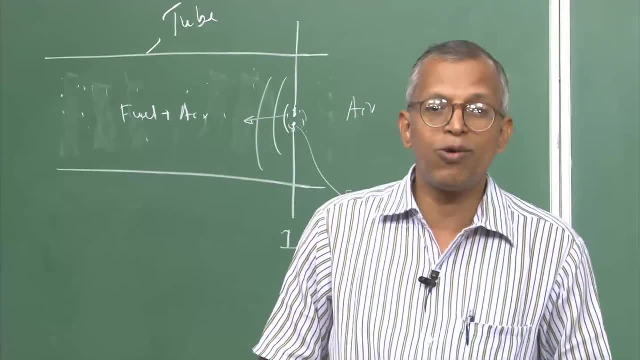 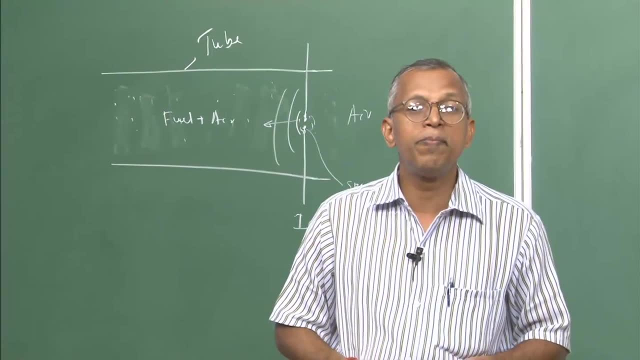 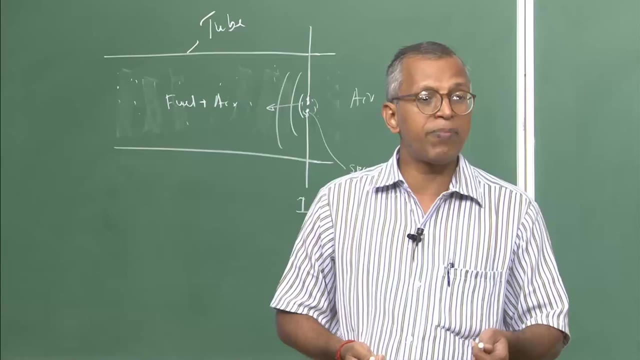 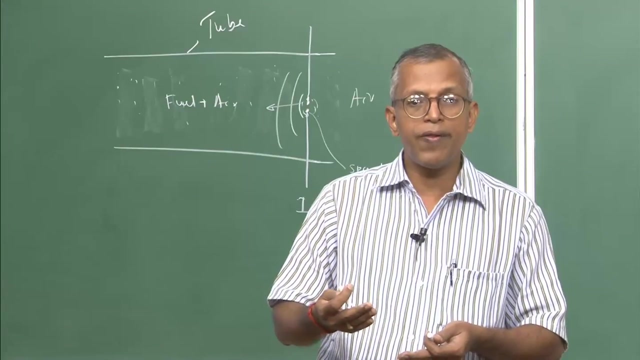 I right, But why it will move at all? what makes it to move? because fuel, air, air is there. is it the reason, then? how does it really takes place? right, because what will be happening? like when the you know flame is formed or flame kernel is being formed, then some heat will. 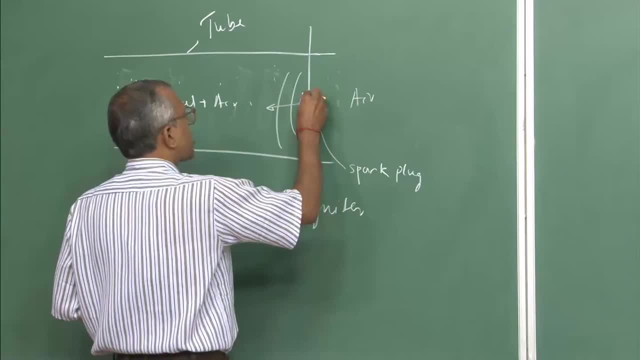 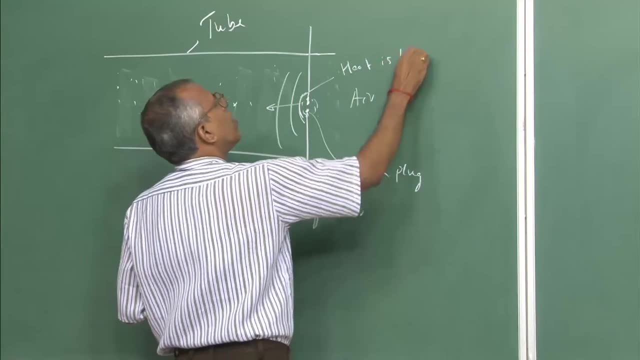 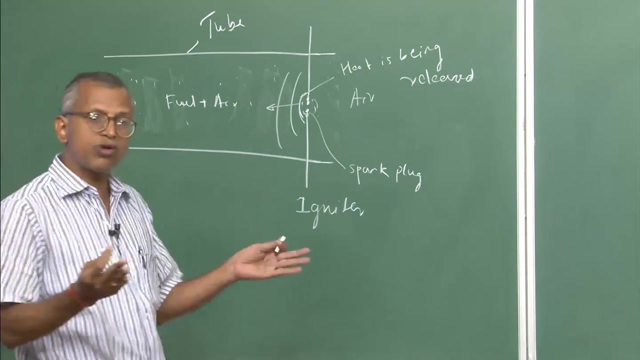 be transferred. right. If it is some heat, chemical reaction is taking place, right, some heat will be released. is not it some heat being released, yes or not It heat being released, then it has to go both the side. it can go this side, it can go this. 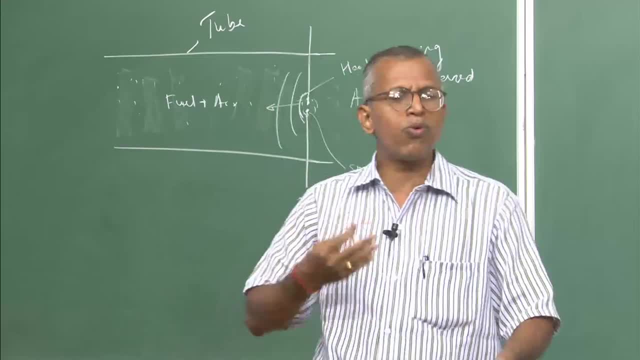 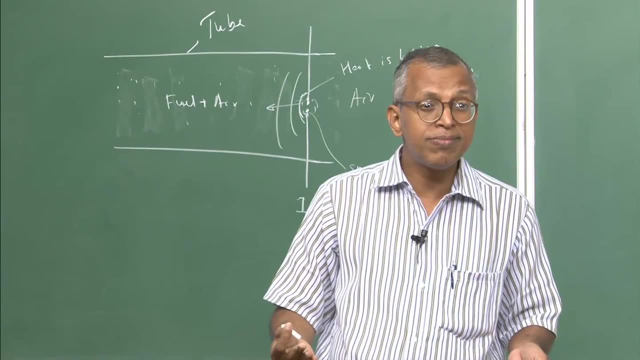 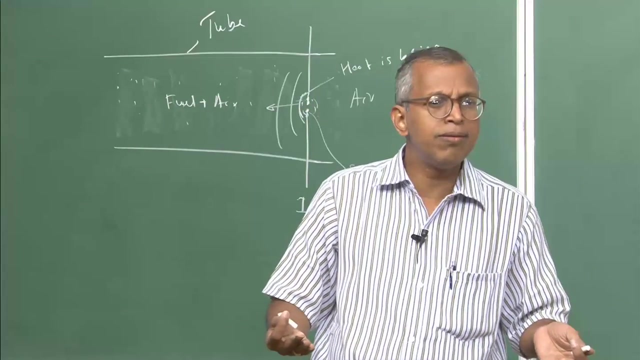 the other side as well, am I right? that depends upon what is the mode of heat transfer, What kind of mode of heat transfer you one can think of. one is conduction, other will be radiation, what else? other will be What else? What will be? convection? right, but is it? convection will take place in this because, keep in mind, 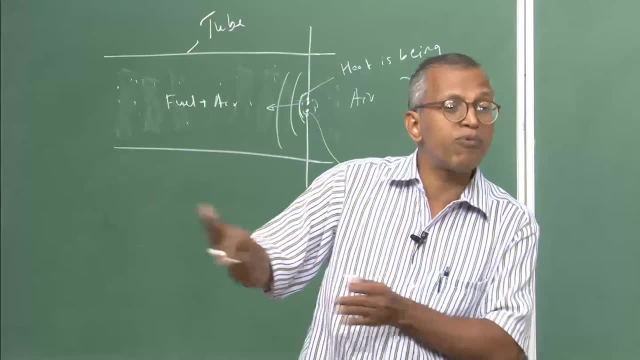 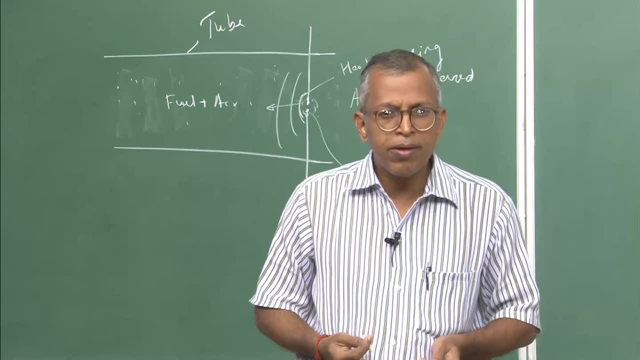 in the tube. the mixtures are stationary. it is not like a pipe which is moving. we are just keeping mixture stationary, right? Will it be? convection will be there, why not? what about natural convection? there would not be any force convection, but natural convection. 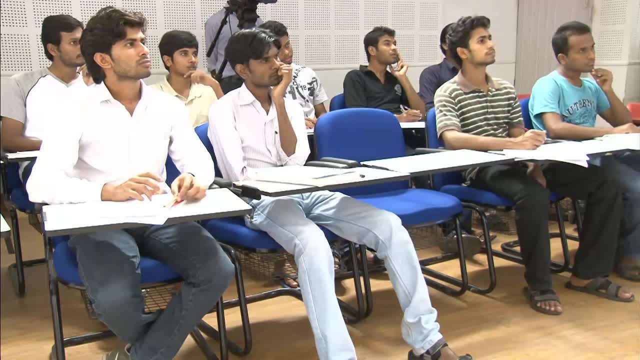 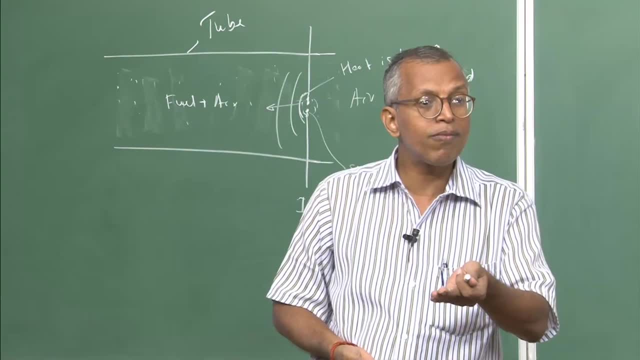 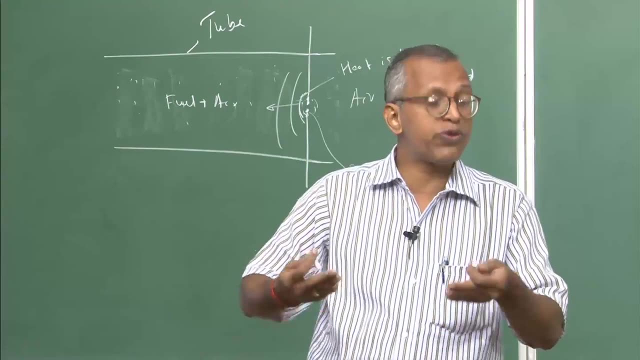 will be there, yes or no, Because if something is hard, that gas will go up because of gravity, right, yes or no? I think you people are not getting. natural convection will be there. radiation will be there because it is very high temperature. you know that radiation heat transfer is proportional. 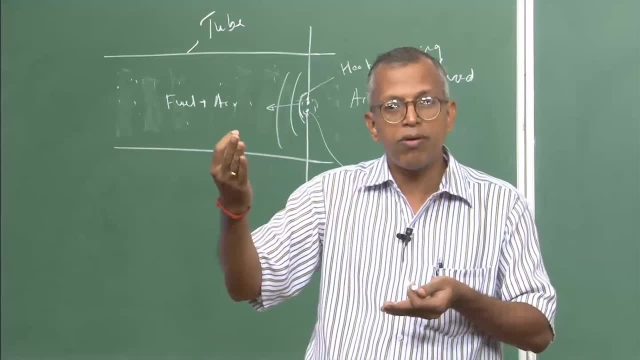 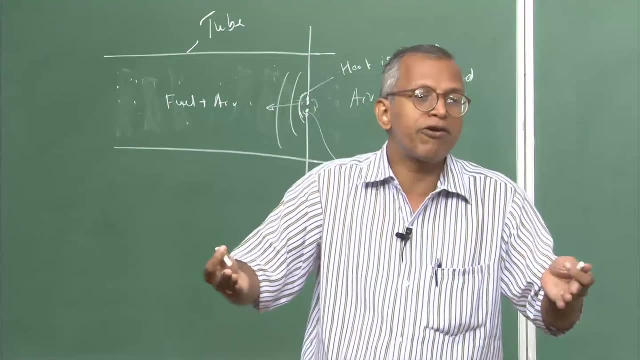 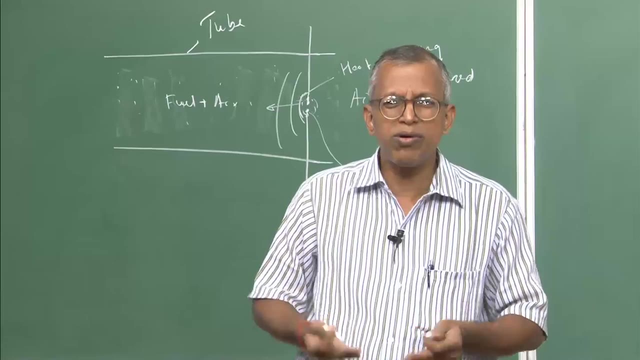 to the power of temperature, power to the four right. So naturally it will be there because temperature is quite high. but in the low temperature I cannot really consider, I need not to consider the radiation If I, If I, If I, Because temperature is effect is not very low, you know right, but at the high temperature. 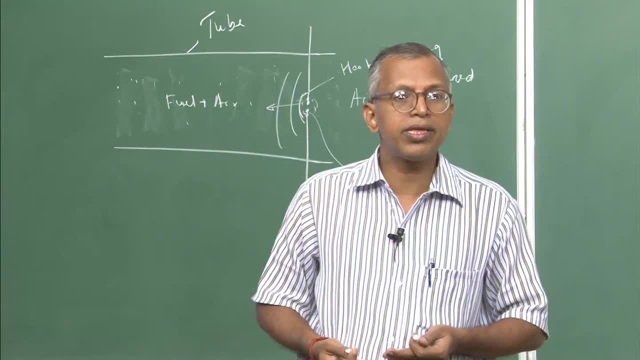 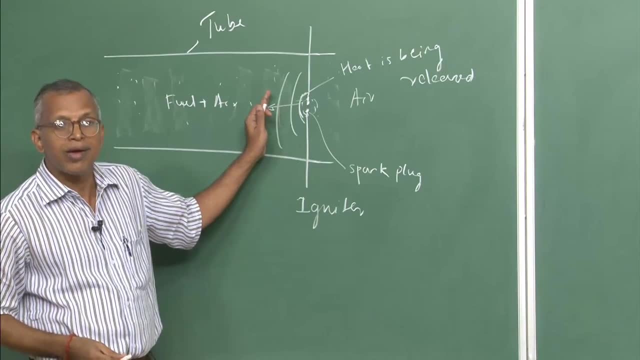 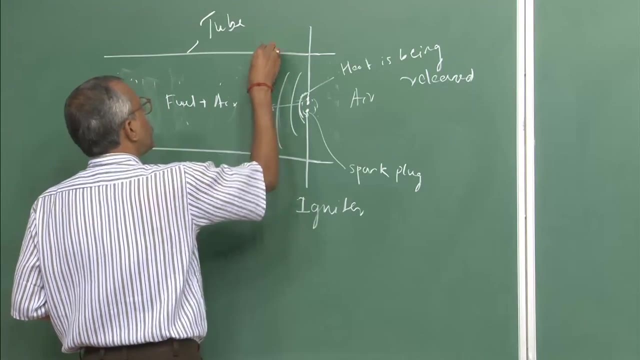 I cannot manage to neglect. it is that clear? So heat will be transfer. if it will transfer, what will happen to the mixture here? its temperature will go up. if it will go up. go up means this temperature. if I put a temperature here, this will be going up. you know temperature of this. 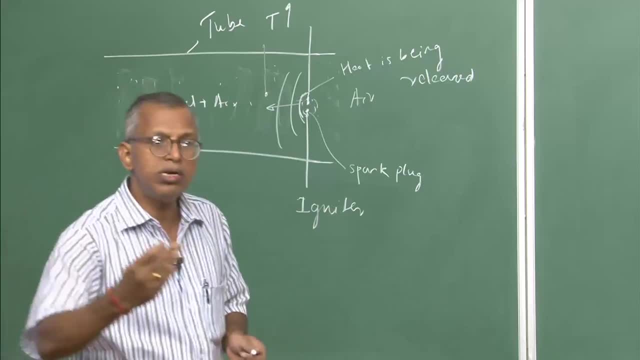 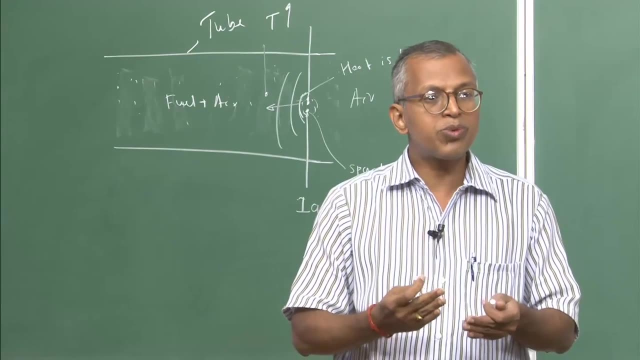 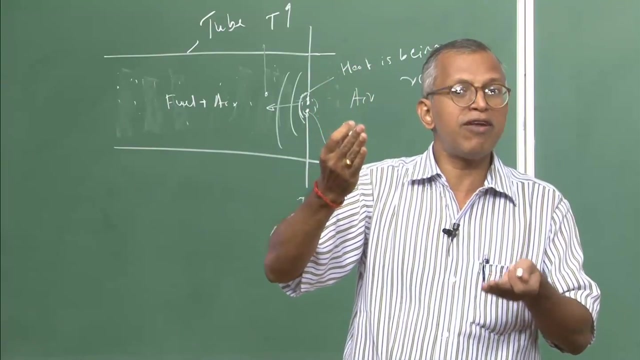 point will be going up, yes or no, Because heat is being transfer. and then what will happen? transfer, then the mixtures temperature will be going up till when it is beyond the ignition temperature, self ignition temperature, then combustion will take place. right, then it will be going, So it will be going at. 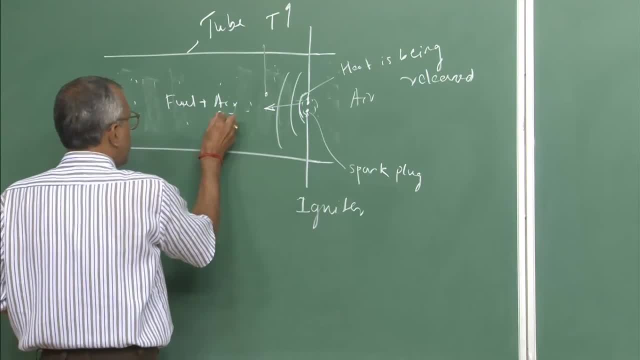 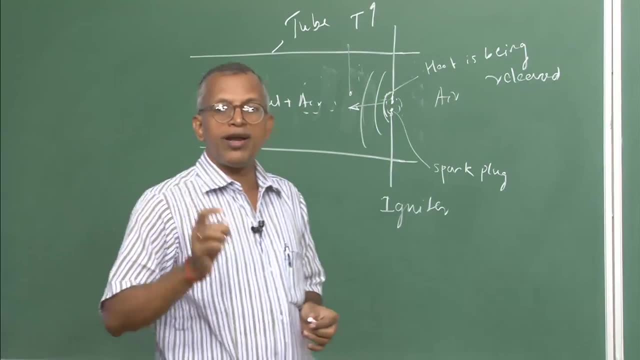 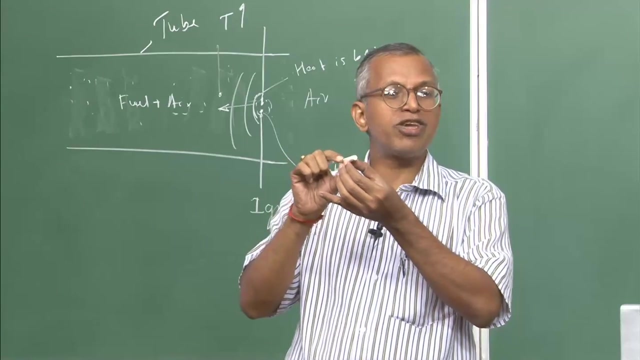 what you call go on moving like a wave in the direction till it all the gases being consumed, right, If you look at you know this example I always give like: suppose this is a food item. let us say there is an insect. you know it will go on eating because, of course, as long as 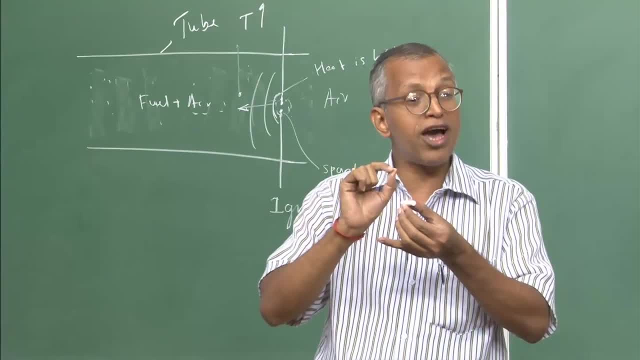 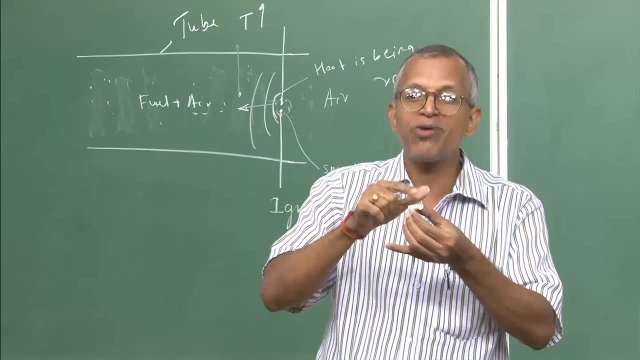 he is hungry. So similarly in our scripture people says that fire is having a hunger to consumed the fuel area, right. So similarly it is go on going, moving that wherever food is there, right. If you look at, you know. like earlier days horses are being put like this: 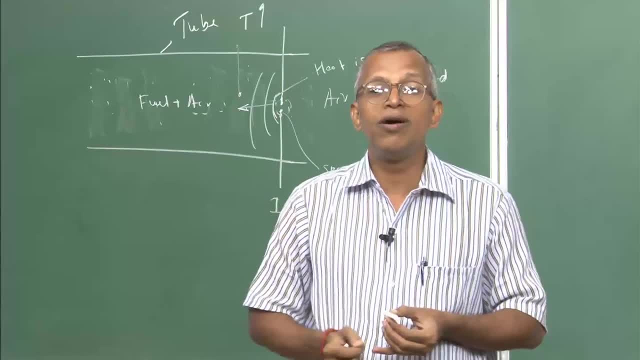 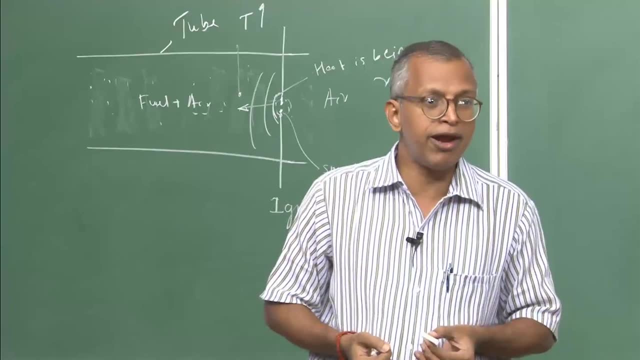 like if they want to make the horse to move. So they will give you the what you call food to lure you by food. like you, people are being lured for getting a job. to study something right, otherwise who will study power? why you are late in class? right, Because you want. 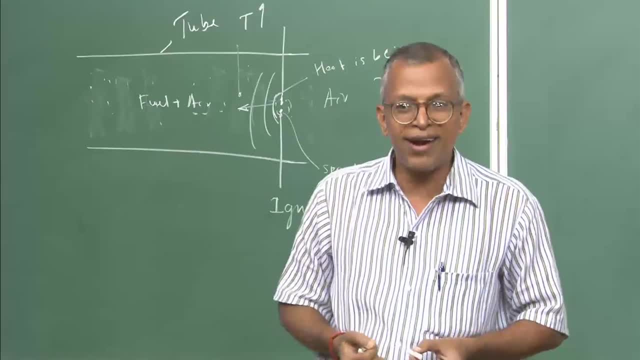 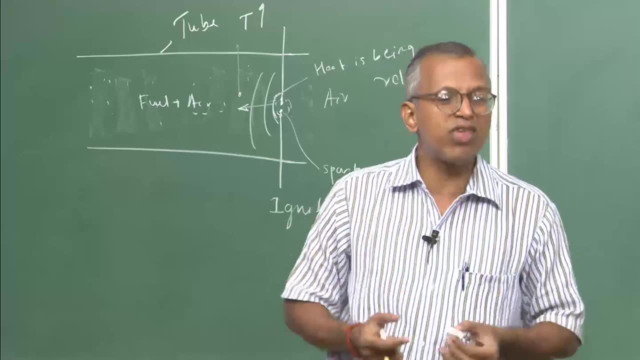 to get a job. that is why you want to work hard and then do that right. It is like that fire or the flame will be trying to go towards the fuel and air. that is a natural way, right? So therefore we will be moving right. 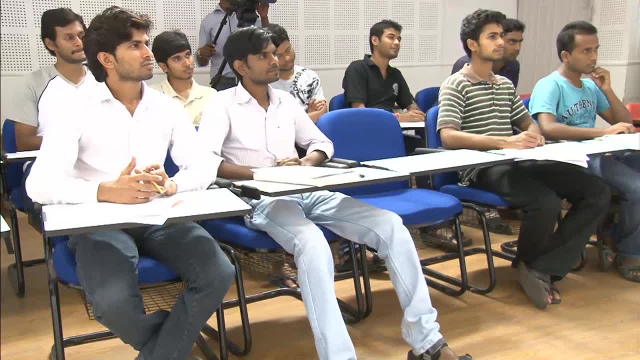 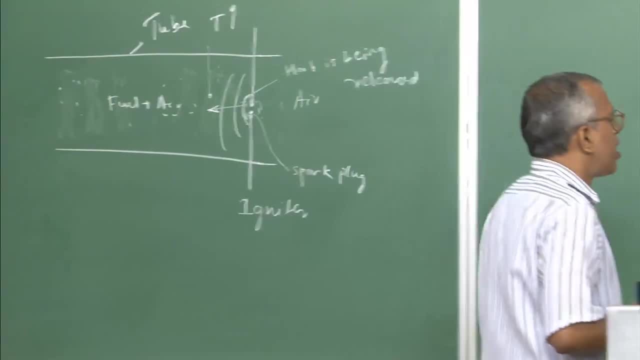 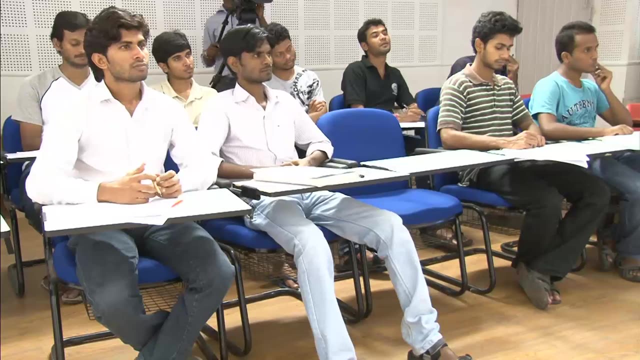 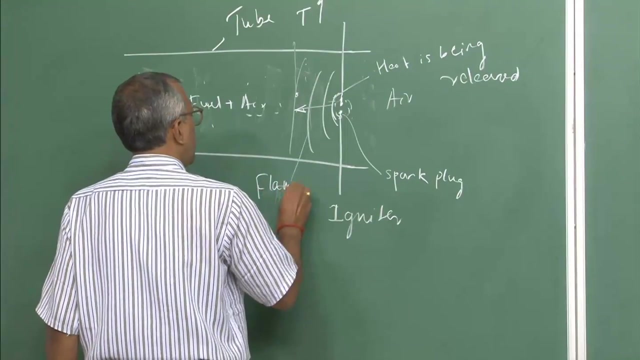 So if I look at this passes, what is this passes? can you give me another similitude which will help you to think better about a flame movement? This is nothing but a wave. it will be moving. it will be moving this flame front. these are flame front, right? These are? 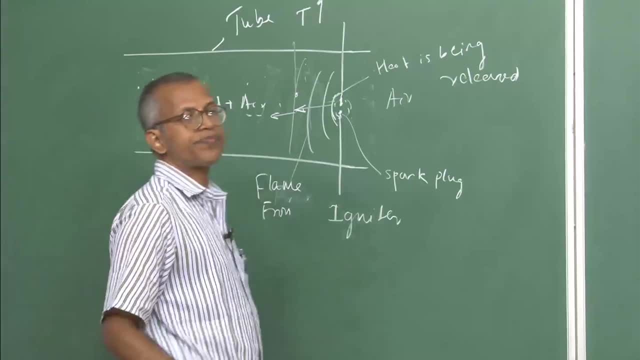 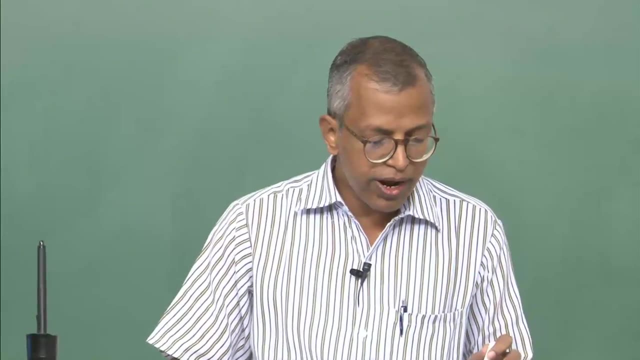 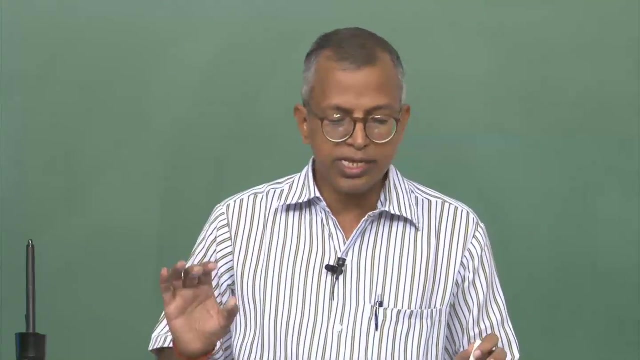 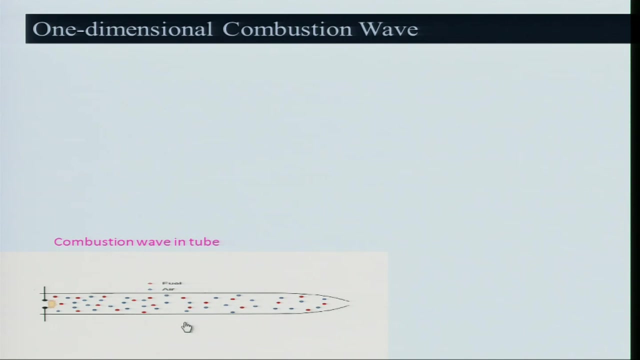 flame front which will be moving right. So now let us look at just that. whatever I have told, let us look at visually what really will be looking at. I have taken a tube, in this case, and there is a tube here, glass tube, where we can, you know, see, visualize the flame. there is ignite, this is a fuel, air mixtures. 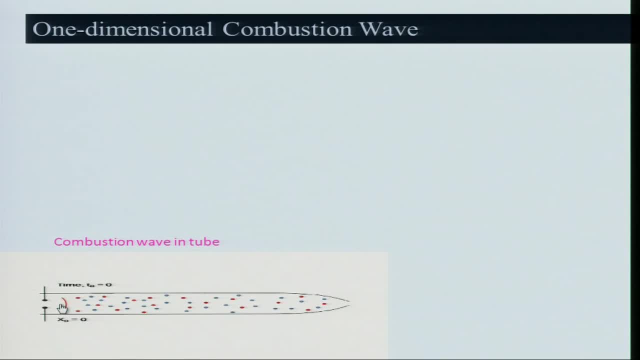 this is ignition, Then what is happening? this flame kernel is being formed, it is moving towards that, it is goes on moving. So if you look at, in the beginning it was like a curve little bit and then this is also flat and, like you know, is a half kind of a moon crescent shape kind of thing. but in 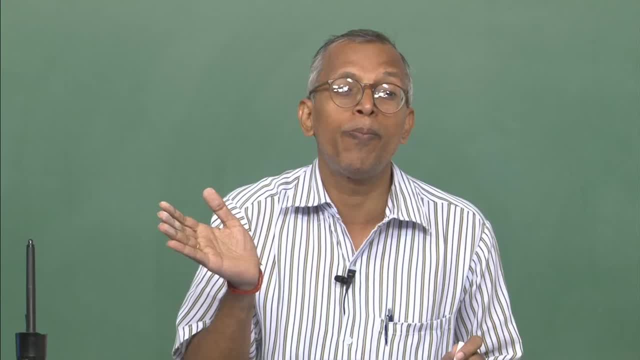 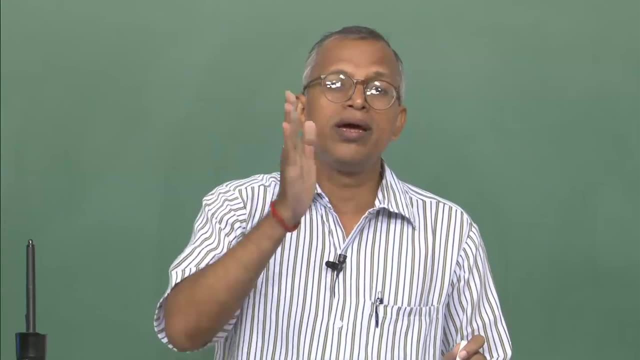 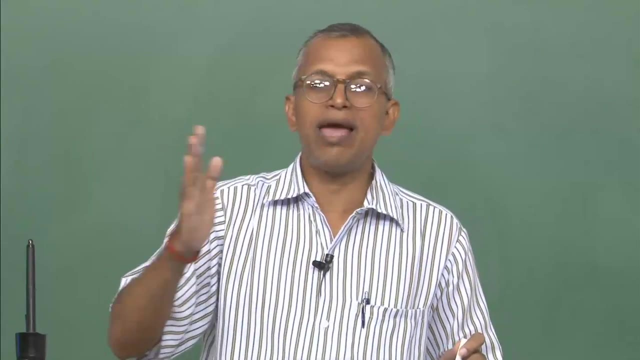 a certain angle, right. Why it is so, why it is not moving as a front, as a- you know, like a little bit curve may be because of heat losses will be there, right- And why it is not moving as a. So this is dimensional, now it is almost two dimensional. why it is so, why it is, you know. 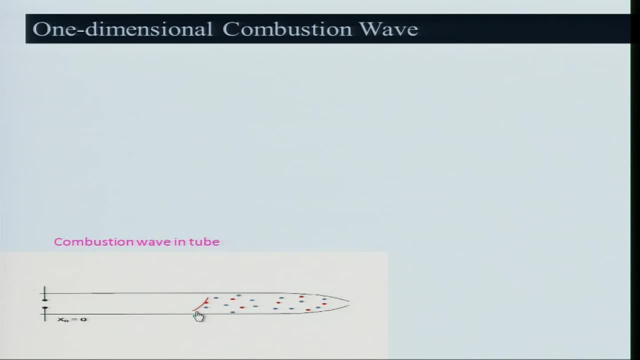 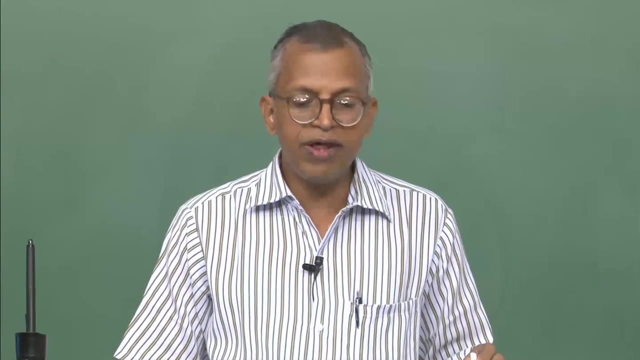 in this region, particularly in this region, it is what you call curve, and then it is you know slanted kind of thing. why it is so? I have already given you an answer for this. because of what natural convection, So? but however, if i want to make this flame stationary, what i will have to do? as a flame? 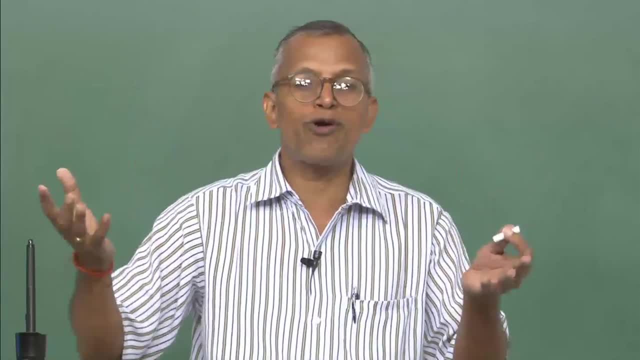 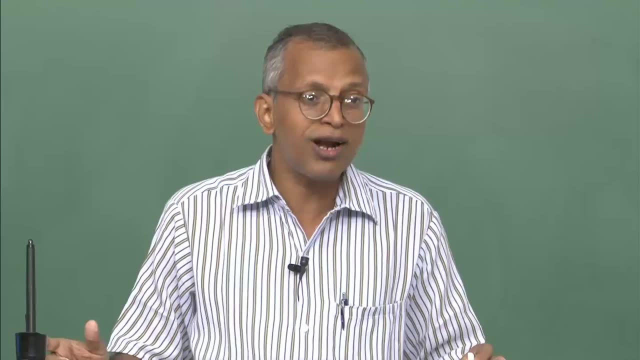 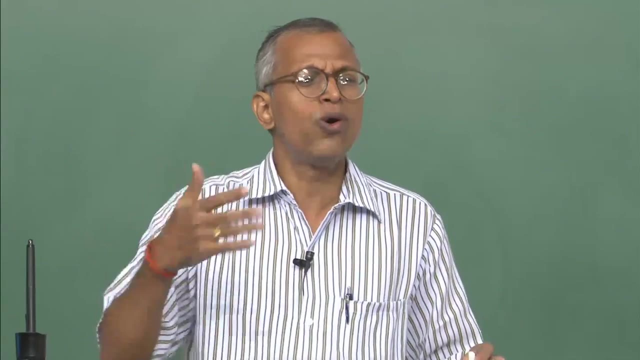 is moving. it is like, you know, fire, open fire goes on moving. you know, you have seen it is devastating, But as an engineer, we do not want the flame to move. we should control the flame such that we can utilize it. that is the whole gamut of, you know, combustors or 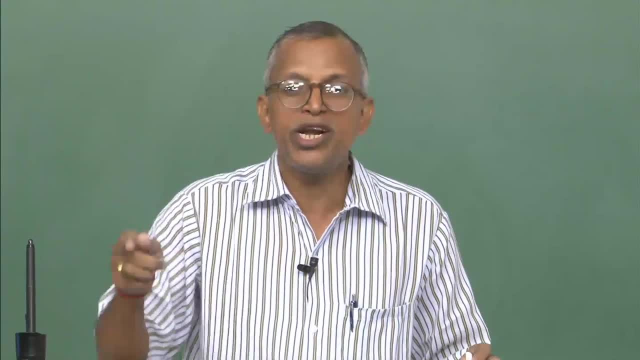 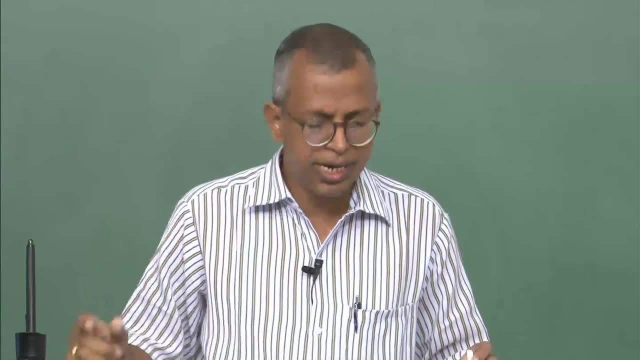 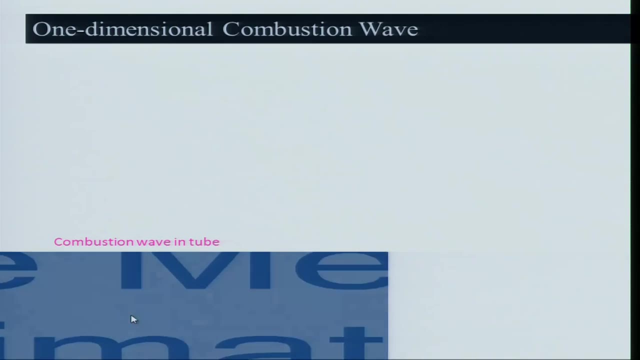 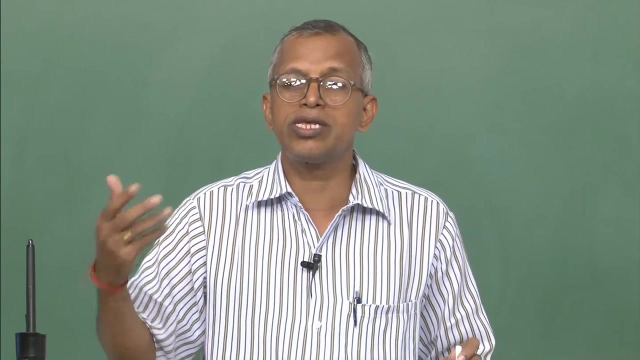 the gas turbine combustors or the rocket engines, we need to contain the flame inside the combustor. For that we need to talk about flame stabilizations and other things. So if you look at like, I want to look at that. So what you do- basically, in this case what you can- I ask you a give. 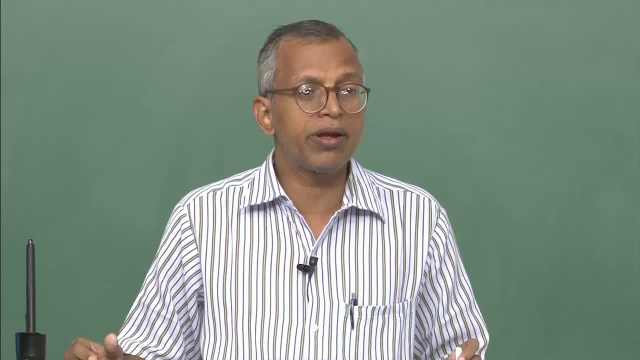 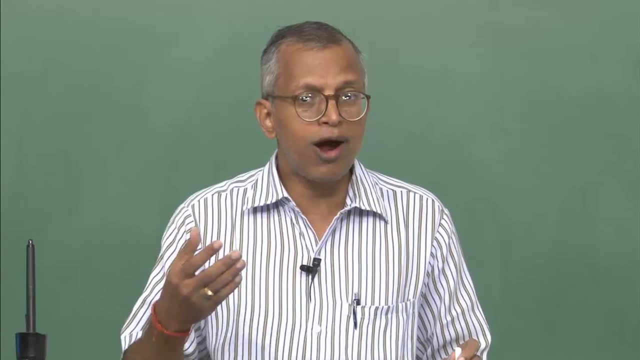 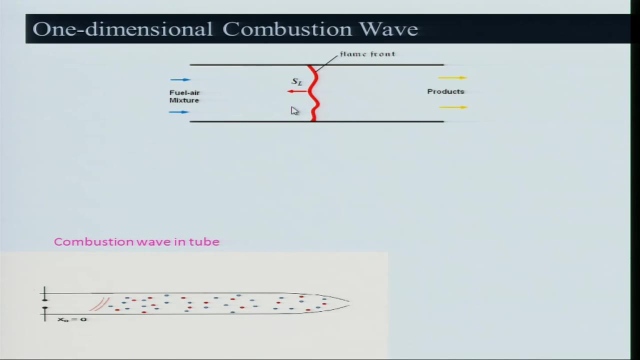 a similitude. what is really happening in this if you look at this example, if you are not thinking about- we will come to that little later on- Let us now look at how we can make it stationary. it is a very simple questions, right, what you 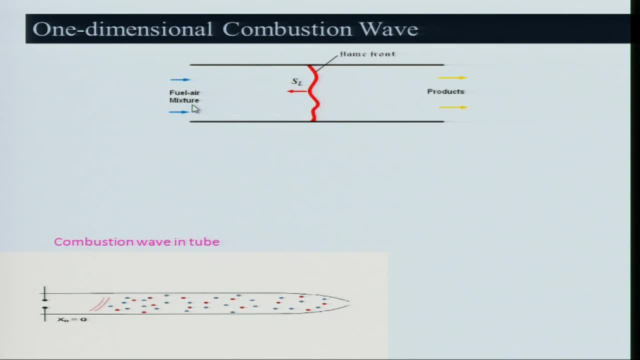 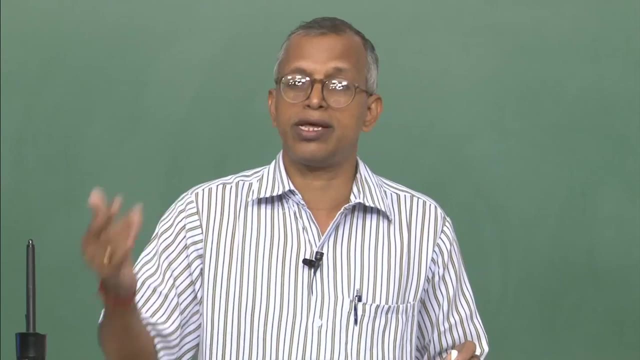 will have to do. I will have to feed this fuel layer mixture with certain velocity with which this flame front will be moving. Like in this case, flame front is moving with respect to, you know, unburnt mixture or the burnt mixture you know, with certain particular velocity. 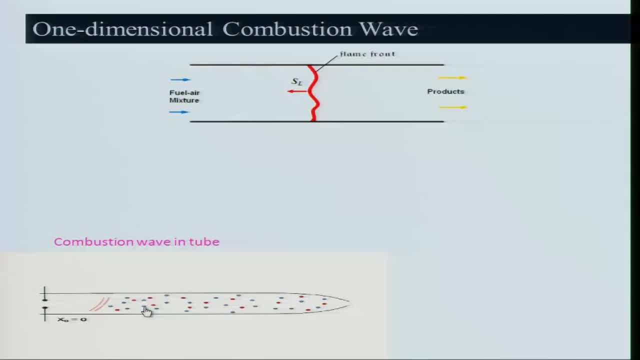 and that will be dependent on what, like I call it, s l, S l is the laminar burning velocity, s l, and it is defined with respect to unburnt mixture. in this case, that means these are unburnt mixtures. right, this is. flame will be moving. 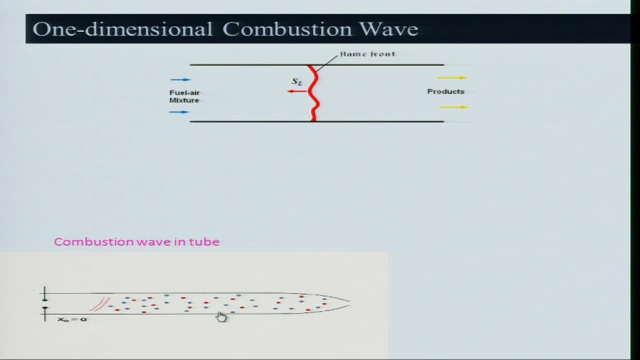 towards this. with respect to this, unburnt mixtures- right then I call it as a burning velocity. Now, if I will allow, if I make the flow right, fuel layer mixture to be flow towards the flame like in the opposite direction of flame. flame is moving in this direction. 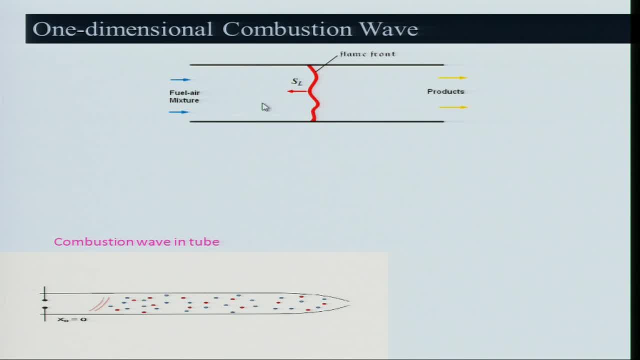 and fuel layer is coming in this direction. if it will be same as that, then my flame front will be stationary. Otherwise, it will be moving either to the left or to the right, depending upon whether the fuel layer mixture is less than the burning velocity or fuel layer mixture. 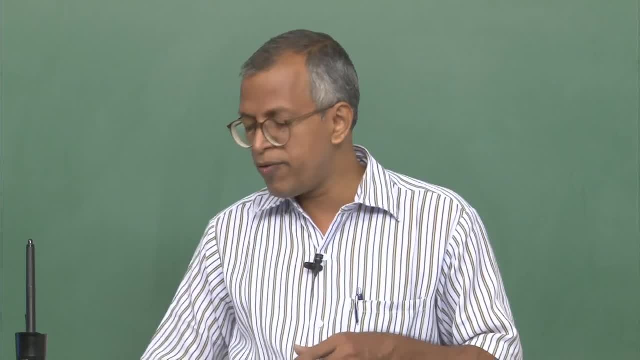 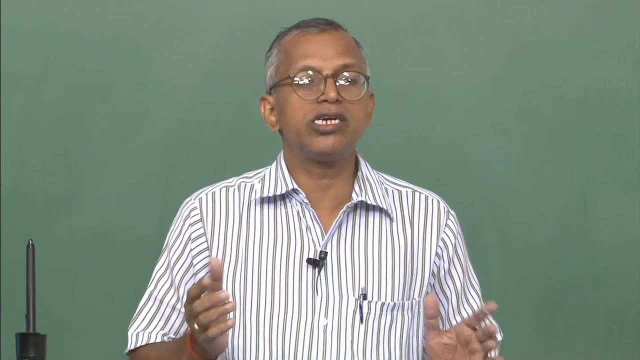 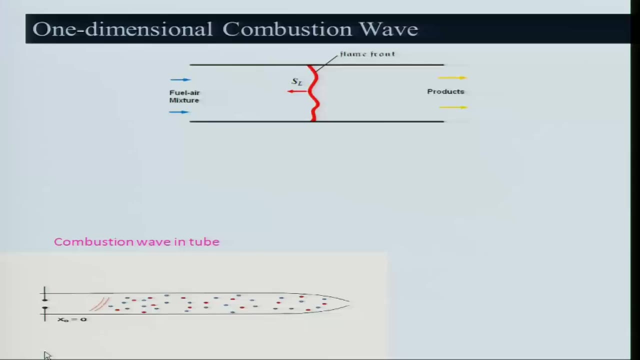 is greater than the burning velocity. this is the basic principle of flame. stabilization is very important point. Are you getting my point? So now, if I will make this, it will be stationary, and if it is stationary, it will be very easy for me to what you call. look at this, one right look. 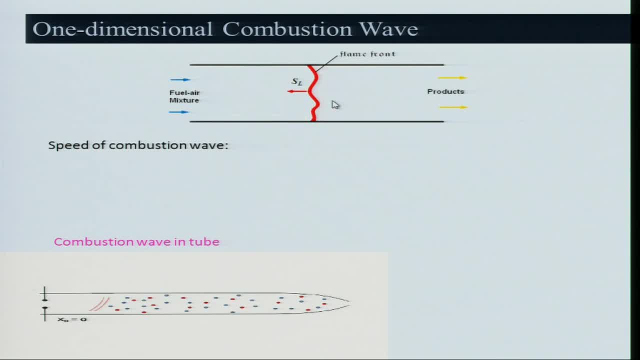 at you know kind of a look at and then analyze. it will do that, like the speed of combustion wave, as I told you, will be varying between two waves: 20 to 340 centimeter per second. keep in mind that if it is a deflagration right, that means 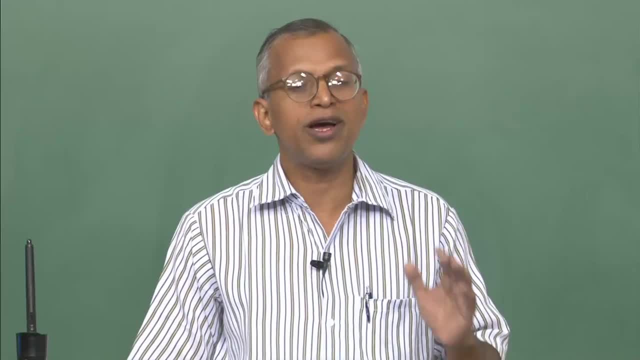 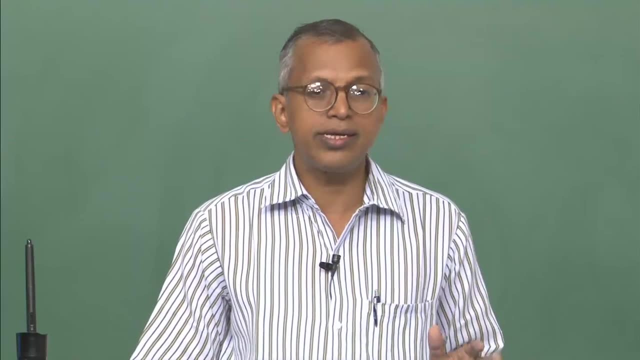 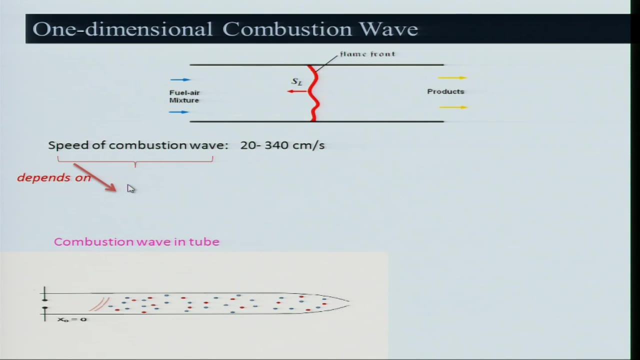 what is the meaning of deflagration? the burning velocity or the flame front will be moving at a subsonic speed, right that we call it as a deflagration right, and it will be dependent what it will be dependent on In late temperature. then what else? fuel, air mixtures, time for fuel layer, like if it is. 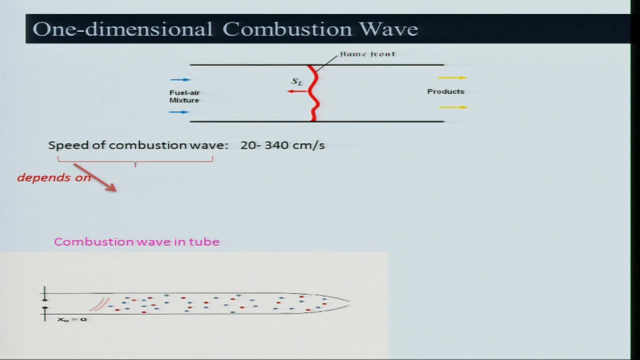 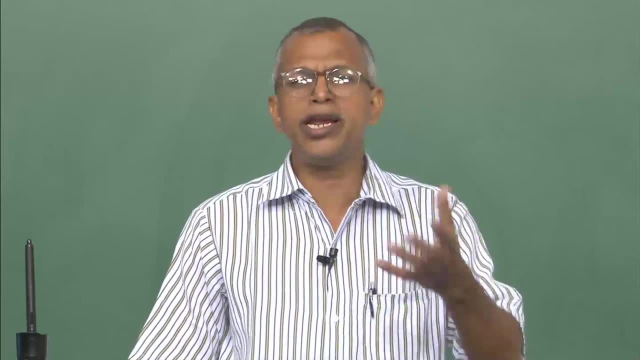 methane air, it will be different. if it is methane oxygen, it will be dependent, it will be. if it is a hydrogen oxygen, it will be different. if it is hydrogen air, it will be different. or any other combination, it will be different, Whether it is a, you know, like a lean mixture. 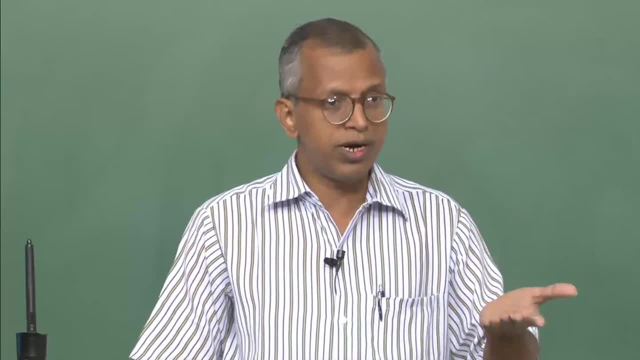 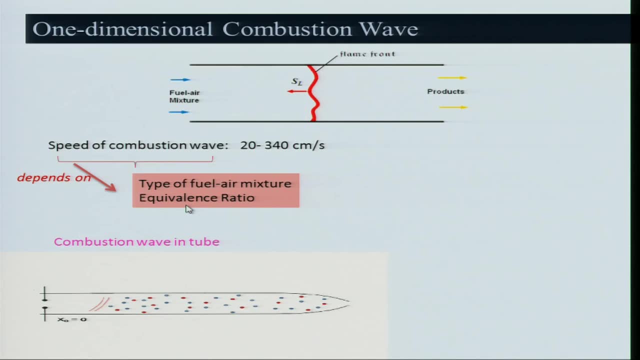 will be different velocity pressure also. it will be dependent on that. so we will be look on, Hit each other vez. Israeli pressure is equal to percent intensity or Wilma's wind. that means it will be type of fuel, air mixtures and other inlet conditions what it would be. 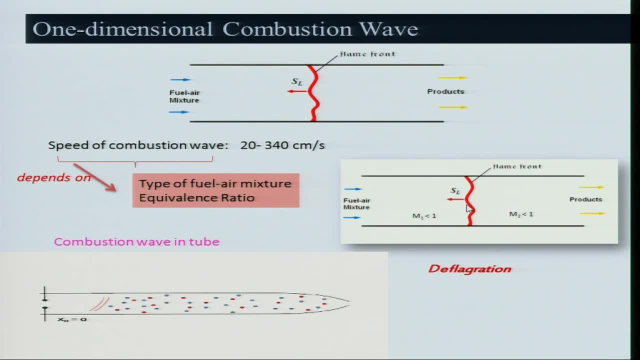 And, as I told you, that, when this flame front will be moving at a, you know, subsonic speed, we call it as a deflagration And I can consider this, as you know, as a one what you call station 1,, station 2, but if this burning velocity, or what you call flame front, is moving at 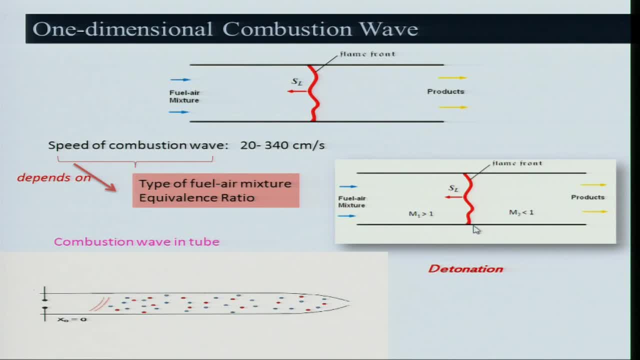 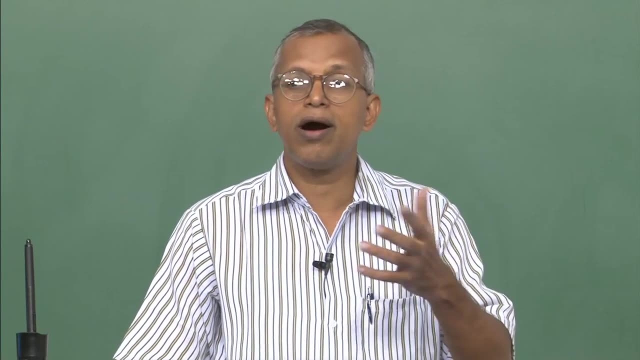 a more than the speed of sound. we call it as a detonation. Detonation is basically a explosion kind of thing, because it is moving at a very high speed. You might have heard, you know, in your, what you call Diwali or the festivals, you know, people make fire cracker. 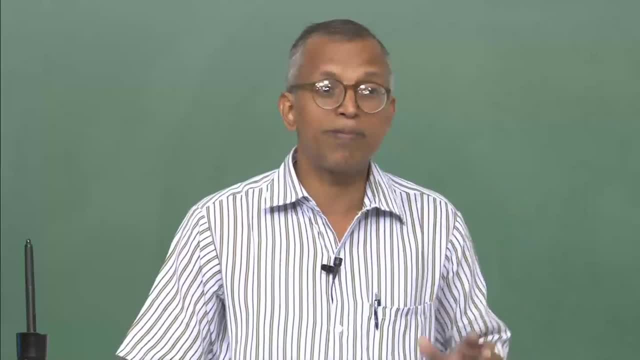 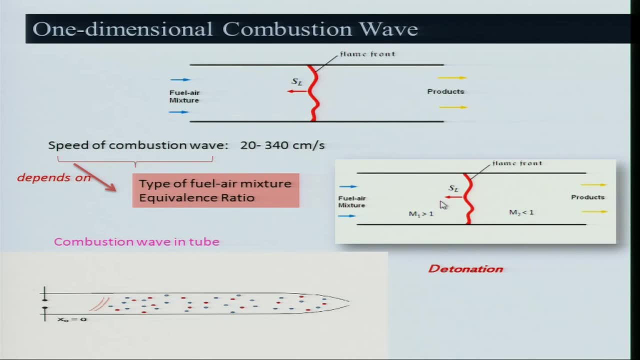 right, Or even like your terrarium Right There is, they put some explosion, you know, like that is a detonation, it is not a deflagration and which is always must be avoided unless otherwise it is useful for the mankind. But unfortunately all explosions and other thing is misuse, abuse for the you know peril or. 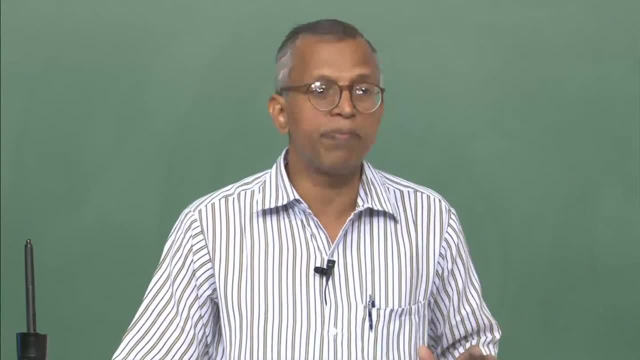 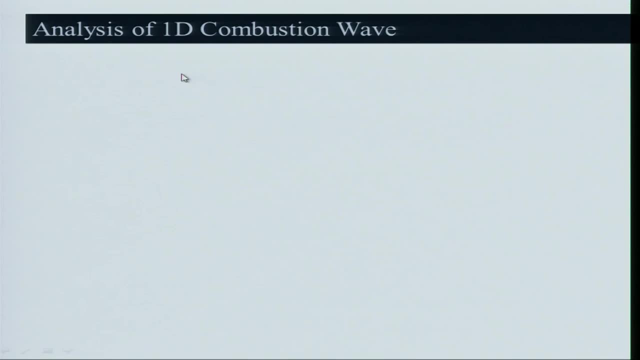 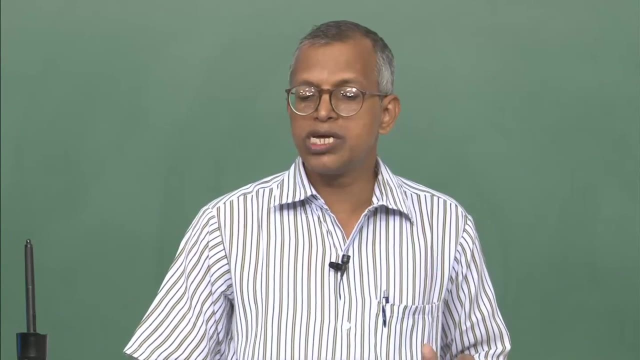 the for the people, you know, against the people. So now let us look at how we can analyze this one dimensional combustion Right, because, as I told you, it is basically wave right and what we will do. we will be using the same continuity and you know all those equation, But what we will be looking, 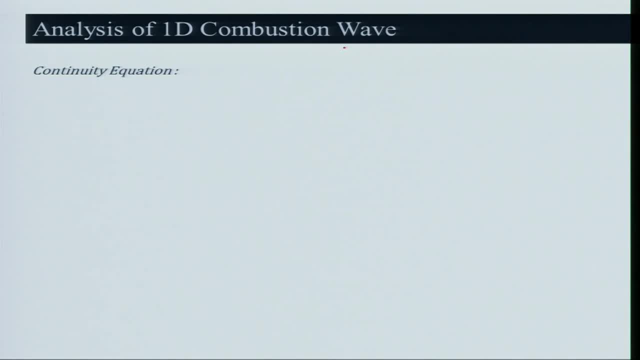 at is like I am having a what you call a tube kind of thing. there is a wave here. you know it is a flame front and I can say this is a 1 and this is 2. keep in mind that this flow is coming over. 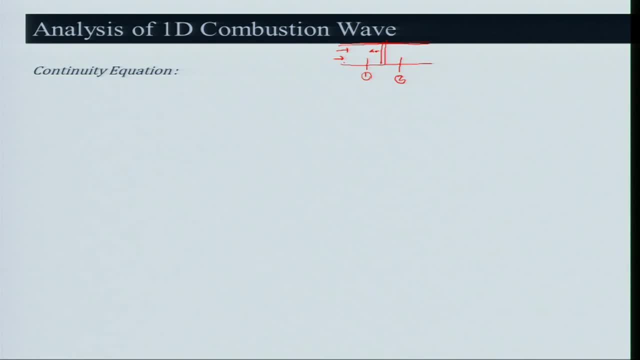 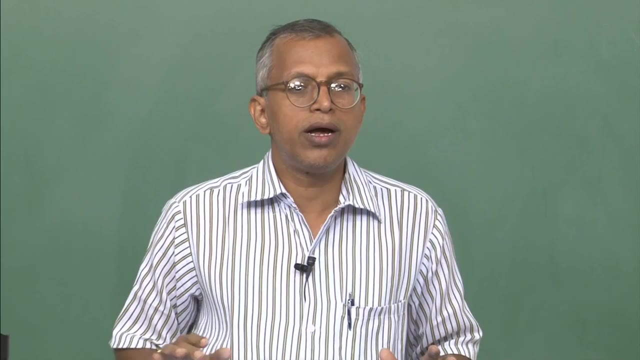 It is moving in such a way. it is moving in some in directions and it is stationary, right, and it is also products are going out. I can say station 1 and station 2. it can be deflagration, it can be detonation, right, We are not distinguishing at this moment. we will be looking, trying to 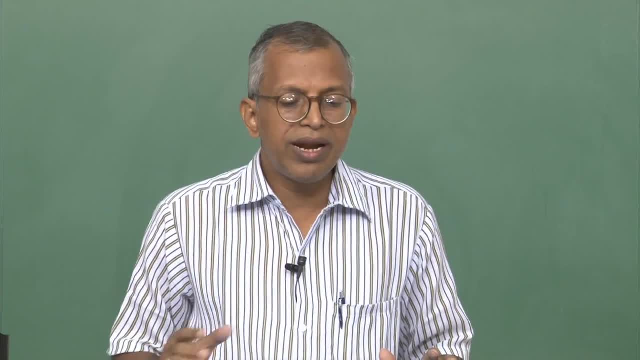 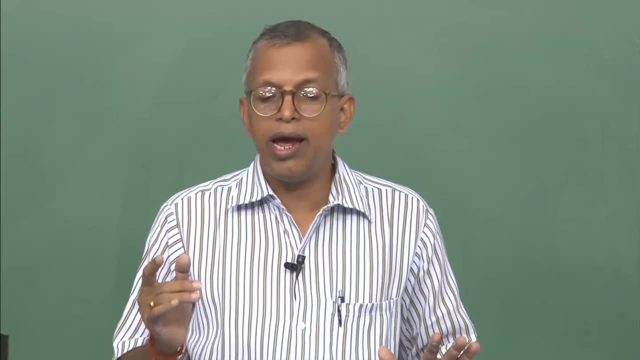 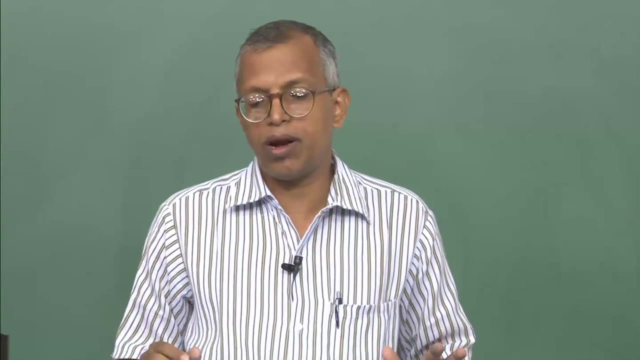 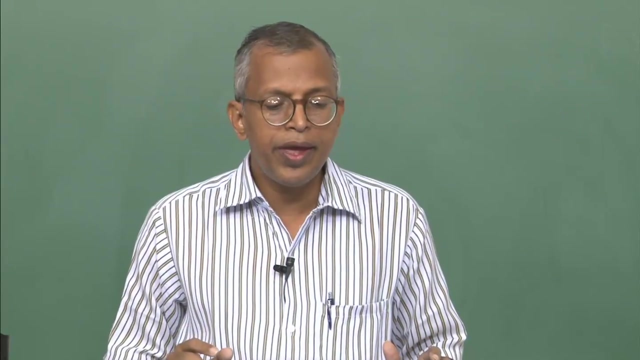 find out what you call the relationship for this and what are the assumption will make will make the steady inviscid flow right And it is basically one dimensional flow right and it is what you call all compressible in nature. flow is compressible because it can take care of both detonation and deflagration.